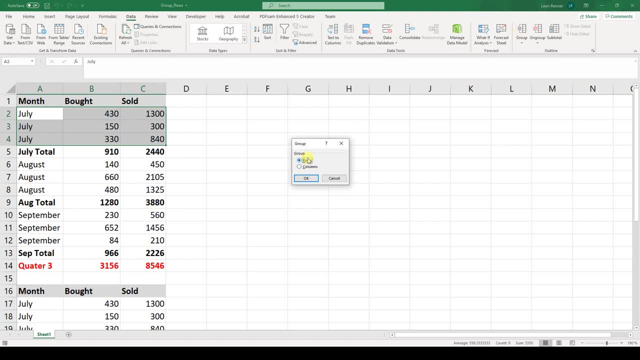 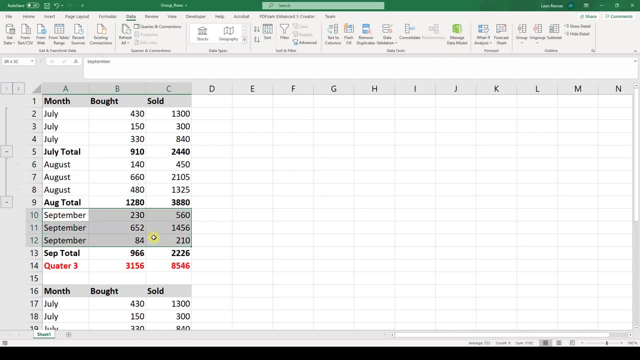 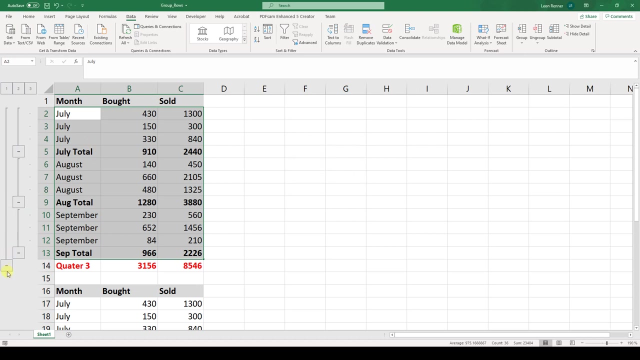 then click on this group button, select rows and click on ok, And you have to do this for the next two group also. And if you now want to create an outer group out of these three months, then simply select the whole group Again, click on group and ok and you can see that you will have an outer group. 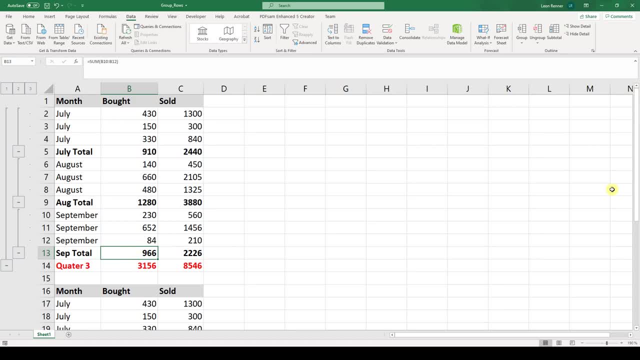 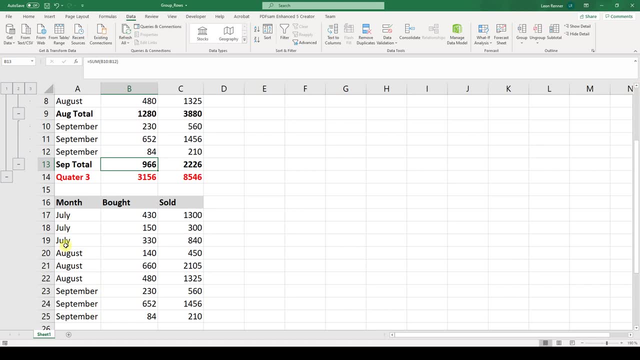 But there's an even easier way, how you can do this, And therefore I copied the whole table here again, And one thing I want to show you is that this table doesn't even contain the subtotals, So you can see that the August total isn't written in here, Since Microsoft Excel will. 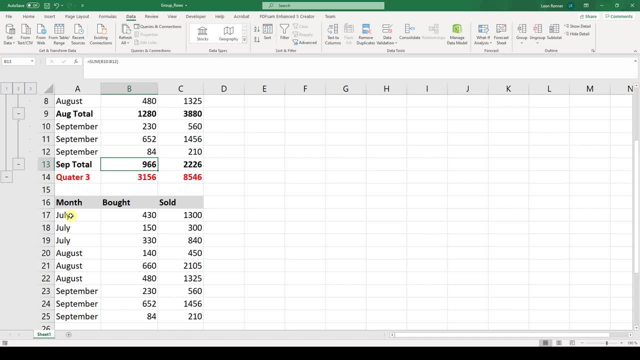 do all of this automatically. So again click in the first cell of your table, But now click on the button subtotal And, as you can see, Microsoft Excel will now create a group basically for each change in the column where it says month. So whenever the value July changes to August, 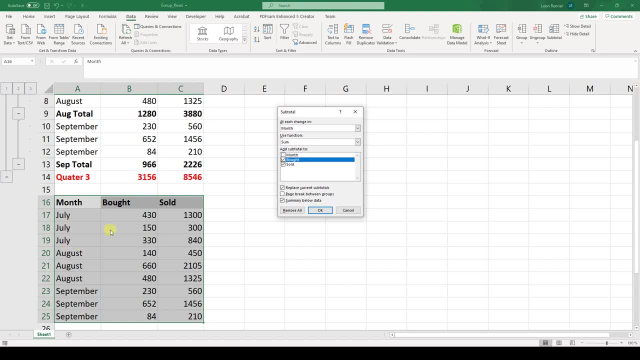 Excel knows that there should be created another group, And the cool thing is that we can now also use a function like the sum function, which basically means that Microsoft Excel will sum up all the values for July, all the values for August and also September. 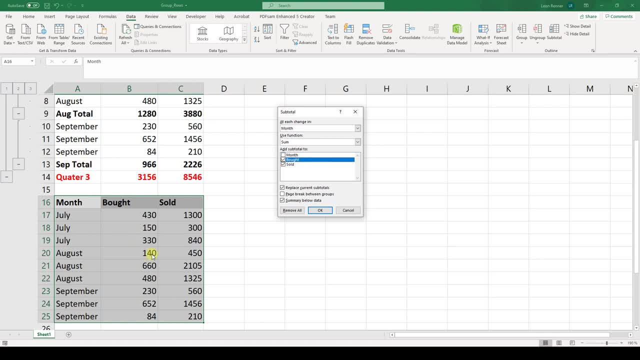 So these totals that we calculated here manually will be done everything automatically. And in this field here, where it says add subtotal to, we simply have to select which columns should be calculated. And since only the bought column and the sold column contain numbers, 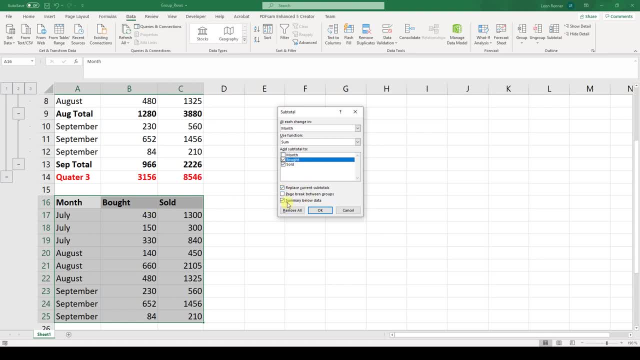 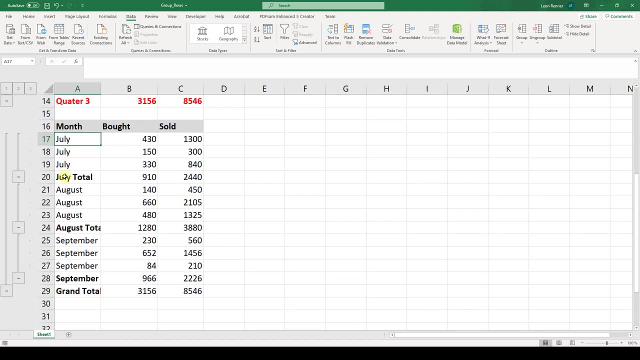 we select these columns here, Then make sure that this summary below data is checked. And now, when you click on OK, you can see that Excel automatically calculated the subtotals, But also integrated the groups. And that's it. Now you know how to group rows in Microsoft Excel.